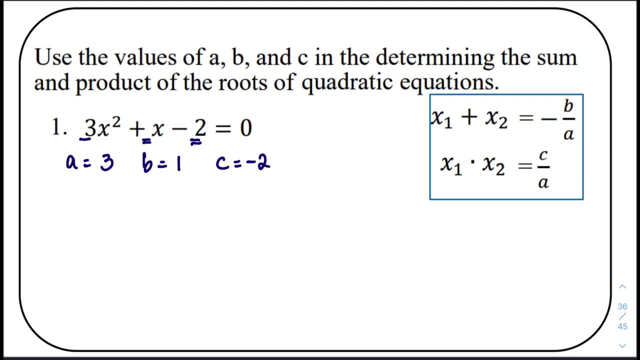 negative 2.. Okay, so, after we can identify the a, b and c, we can now get the sum and product by applying or using this formula: Okay, to get the sum, so that is x sub 1 plus x sub 2, our formula is: we have 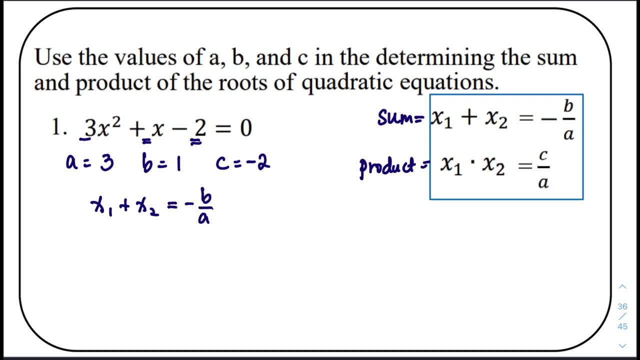 negative b over a. So let's substitute, guys, our b and a here. So we have negative b. So our b is positive 1, right, Then our a is positive 3.. So we have negative 1 over 3.. 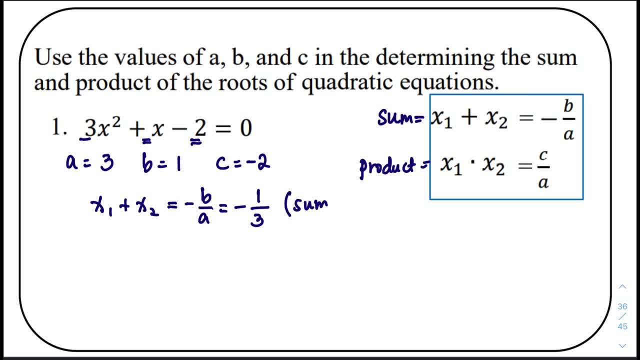 So this is the sum of the roots. Okay, Then, to get the product of the roots. so let's use x sub 1 times x sub 2.. This is the product of the roots. The formula is c over a. 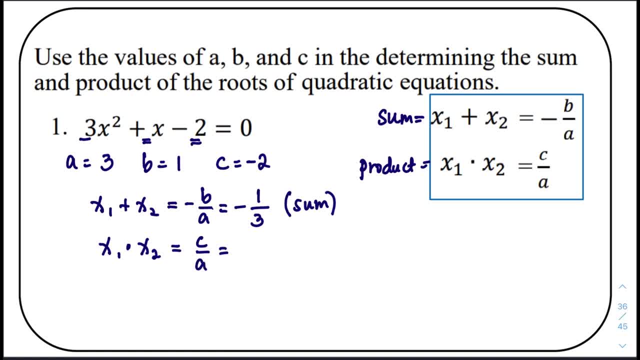 So substitute natin, guys, yung c. We have negative 2 over a. Ang a natin is 3.. So therefore ang product of the roots natin is equal to negative 2 thirds. Nakuha ba guys? 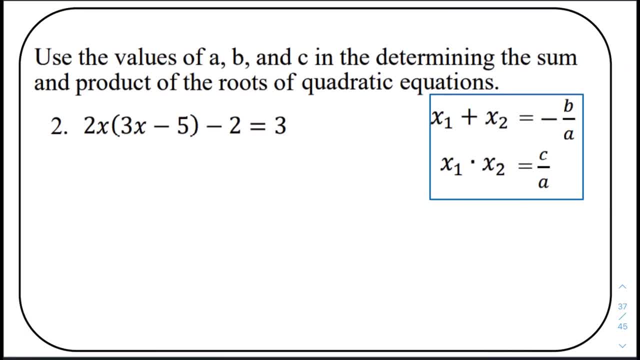 So let's have another example. We have 2x times the quantity of 3x minus 5 minus 2 equals 3.. So let's have another example. So let's have another example. So ang first step nyo, dito, guys, is to rewrite our quadratic equation in standard form. 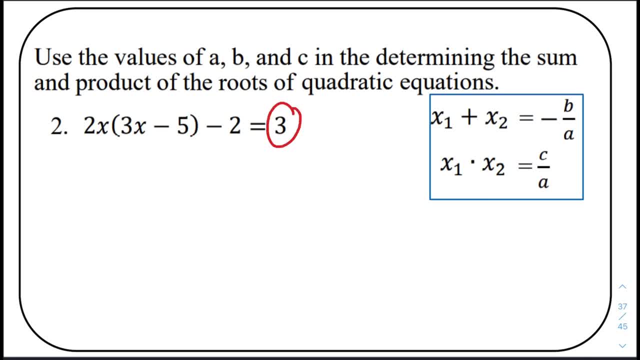 Okay, Then make sure na yung right side ng ating equation ay 0.. So try natin. So first, distribute natin yung 2x. We have 2x times 3x, That is 6x squared. 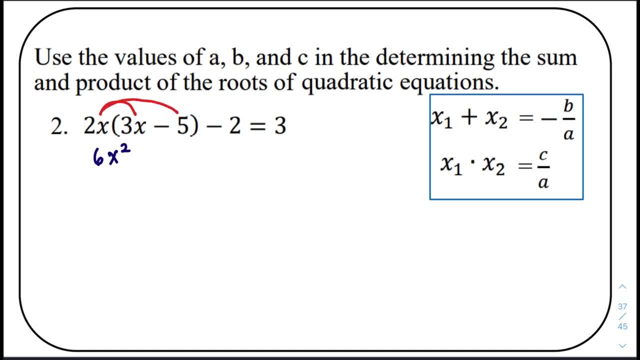 Followed by 2x times negative 5. That is equivalent to 2x. That is equivalent to negative 10x. Okay, And then minus 2. Bring down lang natin yan. So transfer natin si 3 to the left side of our equation. 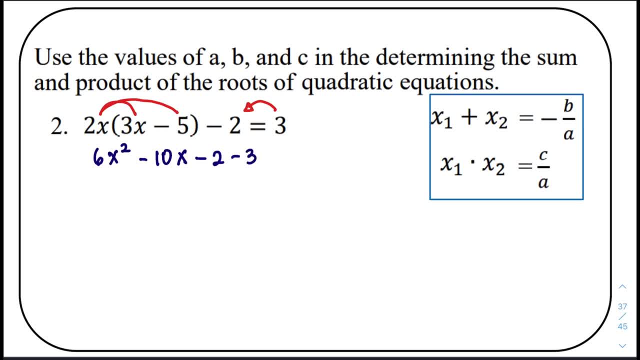 So positive 3 yan magiging negative 3.. Equals 0.. Okay, Then, combining similar terms, So that is 6x squared minus 10x, So negative 2 minus 3.. That is negative 5.. 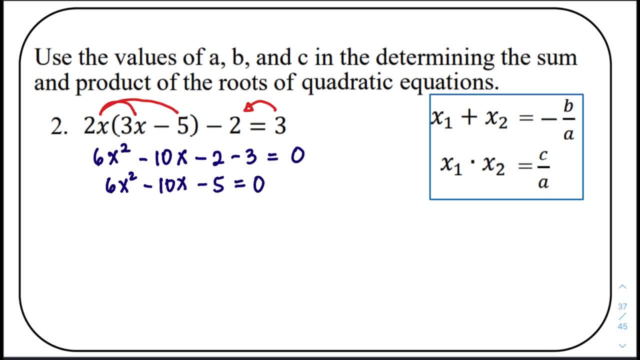 Equals 0.. Nakuwa ba. So after that we can now identify the values of A, B and C. Okay, So ang A natin dito is our leading coefficient, which is positive 6. Ang B natin is the middle coefficient, which is negative 10.. 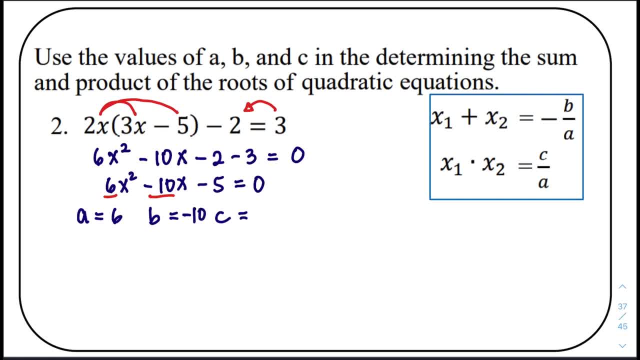 Then last one, ang constant natin, Which is negative 5.. Okay, So, after natin guys ma-identify si A, B, C, pwede na natin makuwa yung ating sum of the roots. 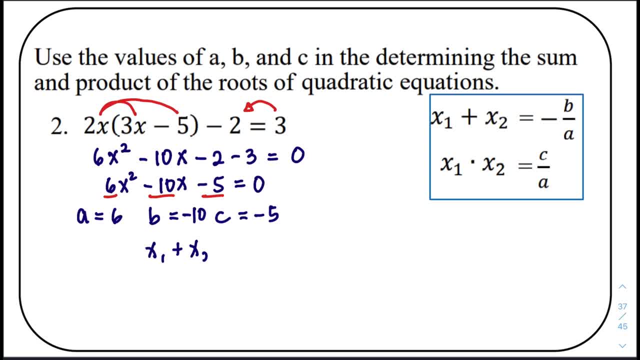 Tama Yung x sub 1 plus x sub 2, ito yung sum ng ating roots, Ang formula negative B over A. So solve natin: We have negative B, So ang B natin is negative 10.. 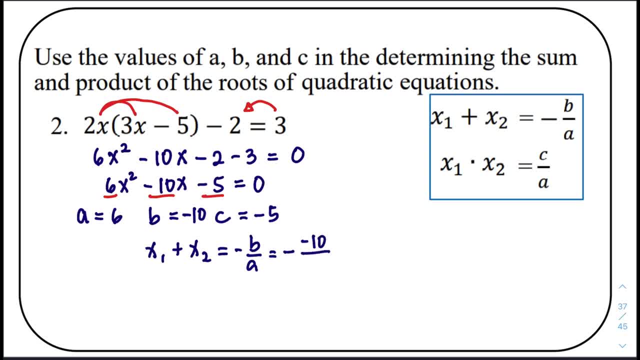 Over A. So ang A natin is positive 6. Okay, Nag-substitute lang tayo. So, kung mapansin nyo, we have two negatives, Ibig sabihin yung sum of the roots natin magiging positive. 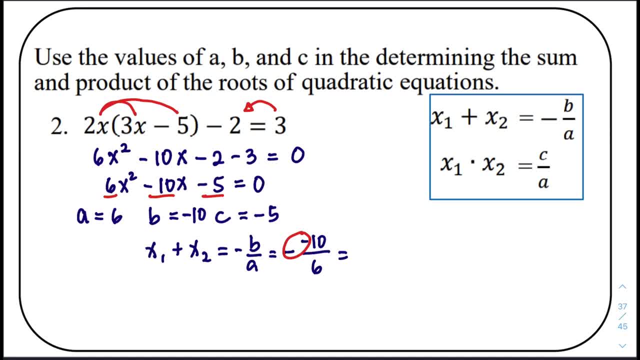 Tama, Since negative times, negative is positive. And then kung 10 over 6 yung ating sum of the roots, Yeah. So lowest term natin, guys, ang gagawin nyo lang: divide natin ito by 2 over 2.. 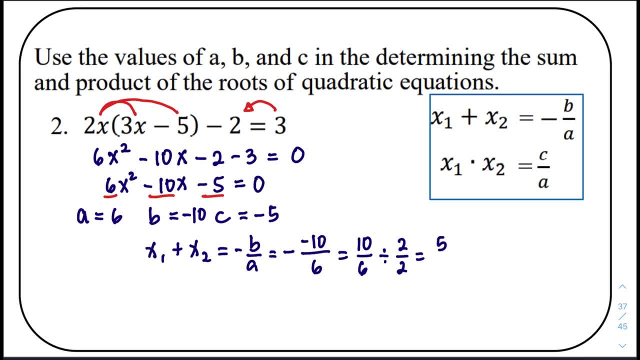 Tama, 10 divided by 2, that is positive 5.. Then 6 divided by 2, that is positive 3.. So ito na ngayon, guys, yung ating sum of the roots. Okay. 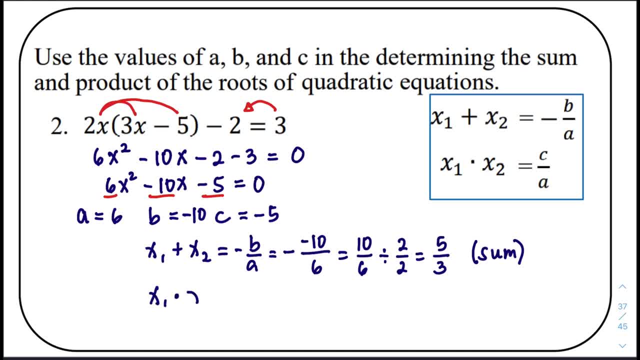 Then to get the product of the roots, i-apply natin yung formula which is C over A. So substitute natin yung values ni C and A. Ang C natin we have negative 5 over A. Ang A natin ay positive 6.. 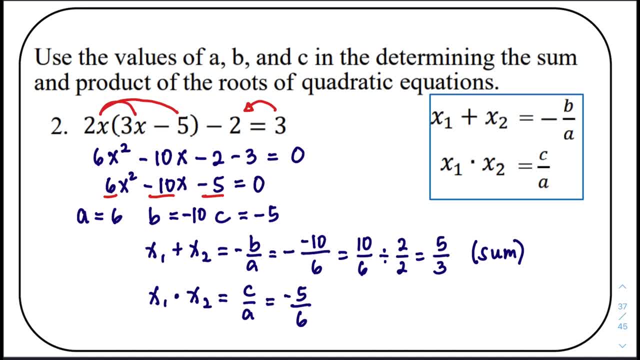 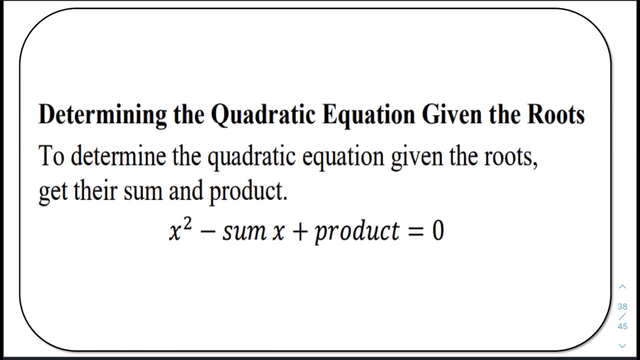 Okay, So negative 5 over 6 yung ating product of the roots Nakuha ba? Okay? So ito na ngayon, guys, yung ating mga final answers. Okay, So now proceed tayo, guys, in determining the quadratic equation given the roots. 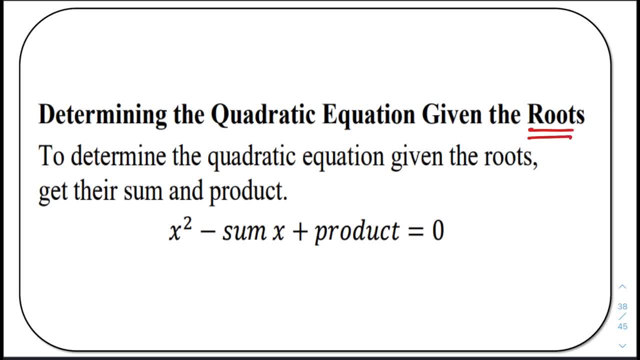 Okay. So sabi dito to determine the quadratic equation, given the roots, get their sum and product. kagaya yung ginagawa natin kanina and then substitute natin guys dito sa ating equation. 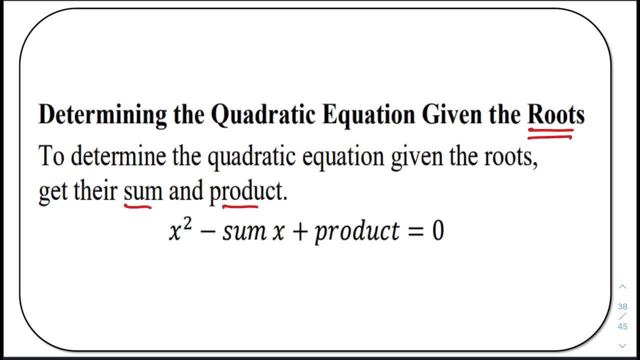 Okay, So ang equation na gagamitin natin, or formula, is: x squared minus yung sum na na-compute natin. then lagay natin yung variable x plus the product ng roots, then equal to zero, Nakuha ba? 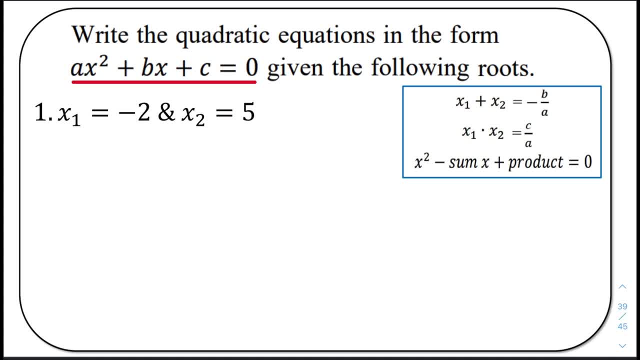 So try natin, guys. So let's have our first example. Write the quadratic equation in the form: ax squared plus bx plus c equal zero. yan yung ating standard equation, given the following roots. So, number one, ang x sub 1, natin we have negative 2, and yung ating x sub 2 is equal to 5.. 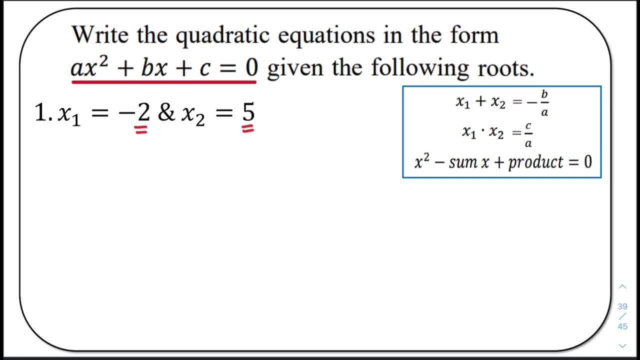 So these are the roots of the quadratic equation. Okay, So first kunin natin yung sum, So that is x sub 1 plus x sub 2.. So ang x sub 1 natin we have. 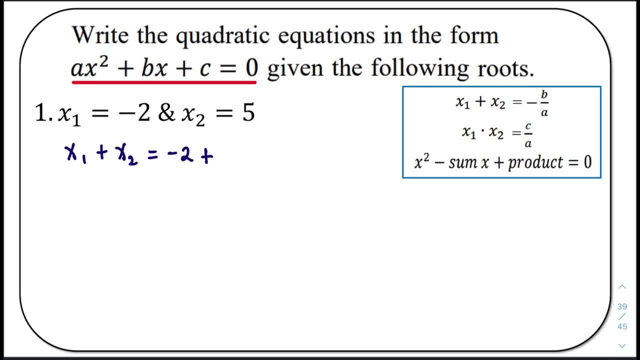 So we have negative 2 plus x sub 2, we have positive 5.. Tama, So add natin to guys negative 2 plus 5.. So that is positive 3.. So ito ngayon, guys, yung sum of the roots natin. 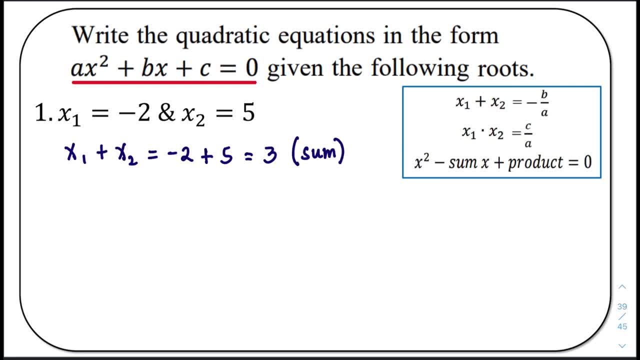 Okay, Then next kunin natin yung product. We have x sub 1 times x sub 2.. So that is equal to x sub 1. We have Negative 2 times x sub 2, which is positive 5.. 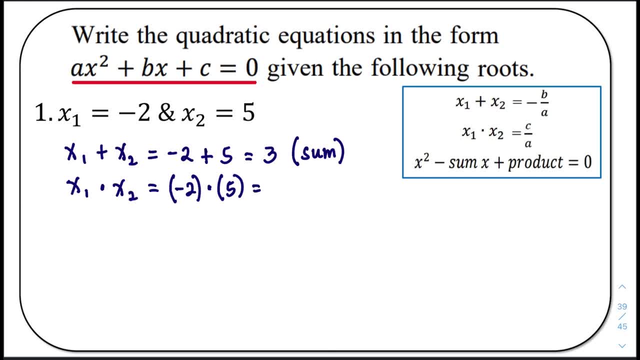 Tama. So simplify natin yan: Negative 2 times 5,, that is negative 10.. Okay So, since opposite yung sign, ang sagot natin ay negative. So this is the product of the roots. 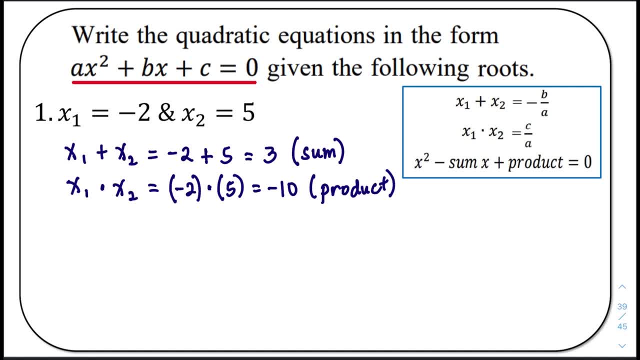 Okay, So after natin ngayon guys makuha yung sum and product ng roots ng kwadrat quadratic equation, we can now use our formula. So our standard formula is: x squared minus sum, then x plus product equals 0.. 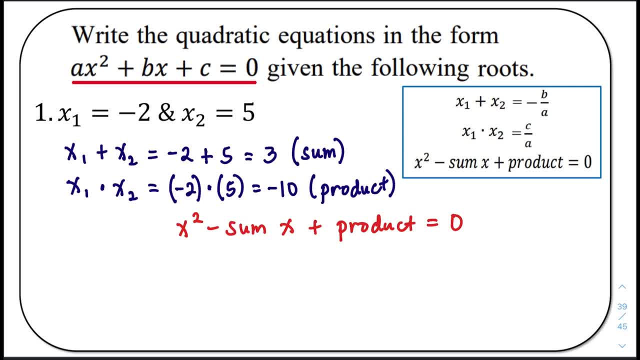 Okay, So substitute natin, guys, yung ating sum and product. So we have x squared minus sum, So ang sum natin is positive 3. Then lagay natin yung x Plus yung product. 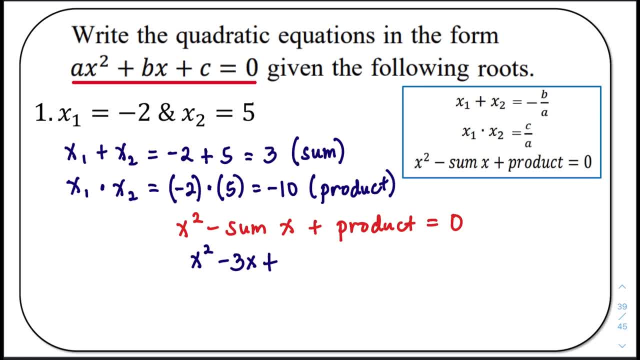 So ang product natin ay negative 10.. Tama Then equals 0.. So, simplifying the equation, we have x squared minus 3x, Then positive times negative 10.. We have negative 10 equals 0.. 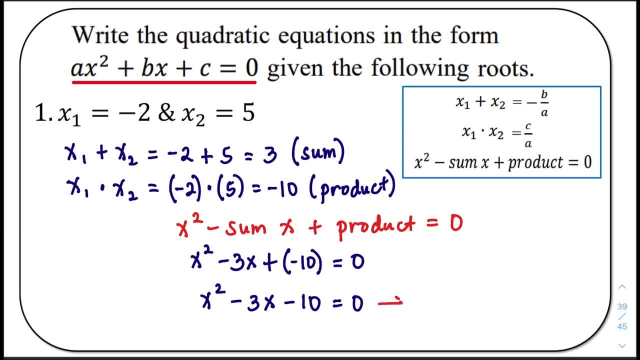 So ito na ngayon, guys, Yung ating Um quadratic equation. Okay, Ang itindihan ba, guys. So let's proceed to another example. We have x sub 1 equals negative, 3 over 5.. 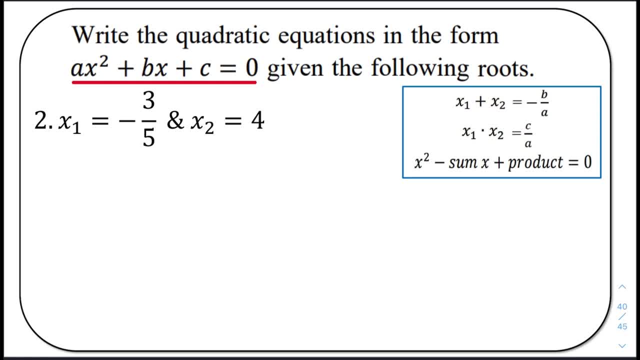 And x sub 2 equals 4.. So again, ang first step natin is to get the sum of the roots, So x sub 1 plus x sub 2.. So ang x sub 1 natin, we have negative 3 over 5.. 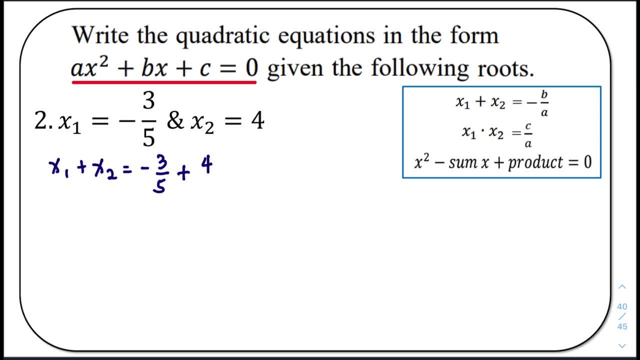 Plus x sub 2,, which is positive 4.. Tama, So, para makapag-add tayo nito, guys, meron tayong fraction. So ibig sabihin, gagamit tayo ng LCD. 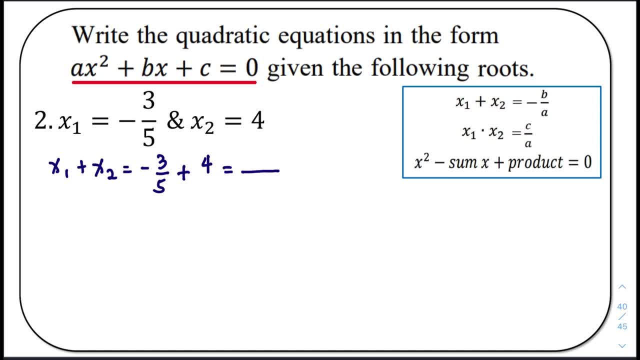 Okay, So si 4 understood yan na merong over 1.. Okay, And then ang LCD ng 5 and 1 is positive 5.. So kunin natin yung numerator: 5 divided by 5, divided by negative 5, that is 1, times negative 3,, we have negative 3.. 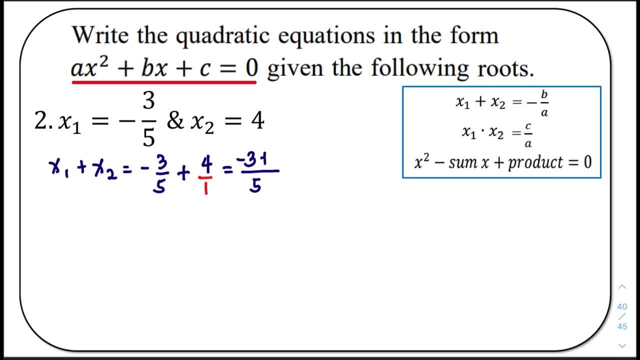 Okay, And then plus 5, divided by negative 1 is positive. 5, times 4,, that is positive 20.. Tama, So combine natin to guys: We have negative 3 plus 20,, that is 17.. 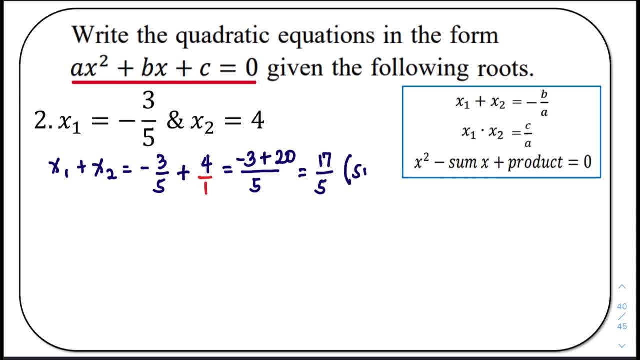 Over 5.. Ito na ngayon, guys, yung sum Okay, And then next kunin natin yung product. We have x sub 1 times x sub 2. So that is negative 3 over 5.. 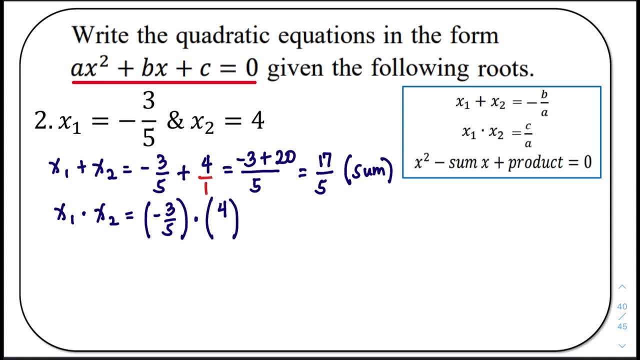 Times positive 4.. Okay, So pag nag-multiply tayo guys nang may fraction. Multiply the numerator to numerator, Then denominator To the denominator, So si 4 dito andres to dyan na may over 1.. 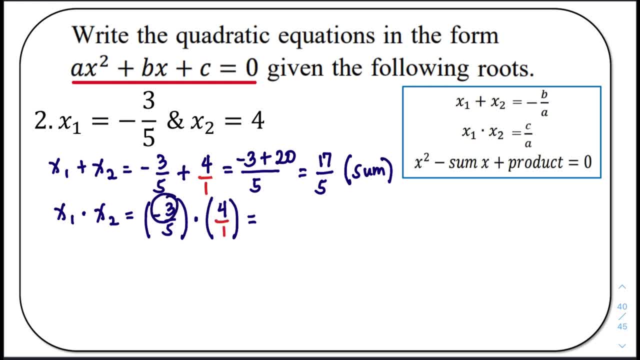 So try natin: Negative 3 times 4, that is negative 12.. Over 5 times 1, that is positive, 5.. Tama, So ito na ngayon, guys, yung product of the roots. 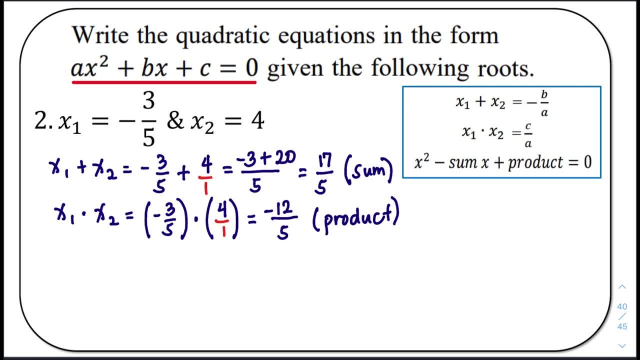 Then after that, we can now use Our formula dito sa may right side ng ating screen To get the equation nung ating quadratic na in standard form. So try natin. So we have x square. 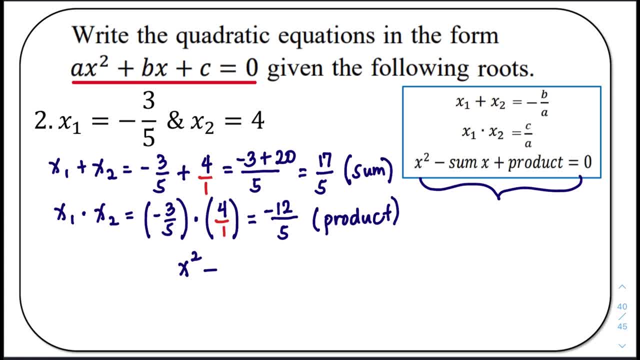 Minus sum, So ang sum natin dito is 17 over 5.. Then lagay natin yung x Dito guys Plus Yung product, So ang product natin we have a negative 12 over 5.. 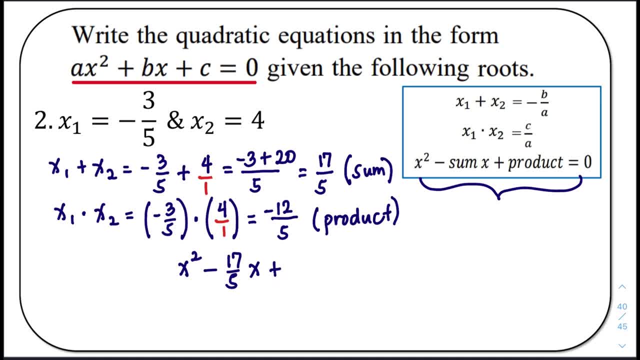 So times natin kay positive magiging minus to Tama. So we have negative: 12 over 5 equals 0. So ngayon rewrite natin yung ating quadratic equation na wala siyang denominator. 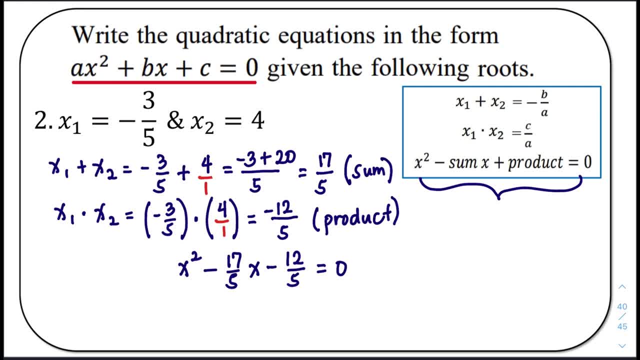 Okay, Para mawala yung mga denominator. kung mapansin nyo, we have 2 denominators, Parehas silang 5.. So just multiply both sides of the equation by 5.. Tama, So try natin.